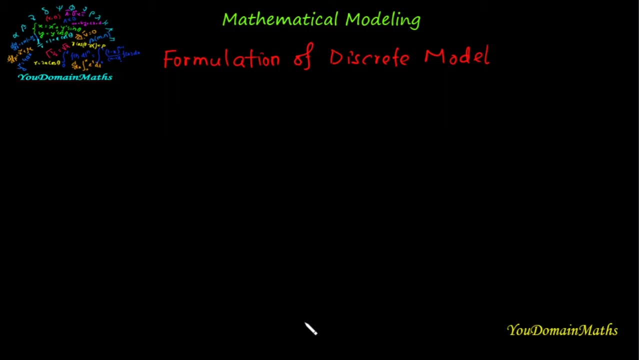 Suppose a cup of coffee- That is a cup of coffee, That is a hot coffee must be Winter. temperatures are 190 degree Fahrenheit, Which is placed in a mold. Suppose it is on the table And the room temperature is 70 degree Fahrenheit. 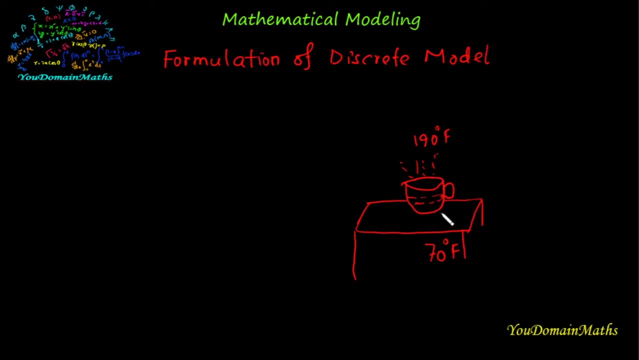 After warming it, the coffee has cooled down. It has cooled to 180 degree Fahrenheit Just after one minute. If we need to find the temperature of coffee after 15 minutes, That means what is the temperature after 15 minutes of coffee? 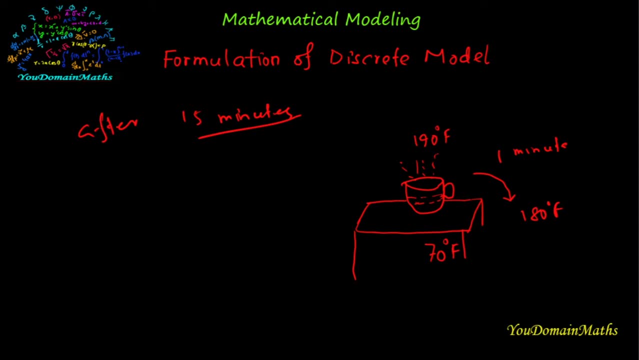 So, firstly, we will find out a relation between present temperature- That means current temperature- And room temperature. We will use Newton's law of cooling. This states that The rate of change of temperature, The temperature of the object, Is proportional to the difference between the room temperature. 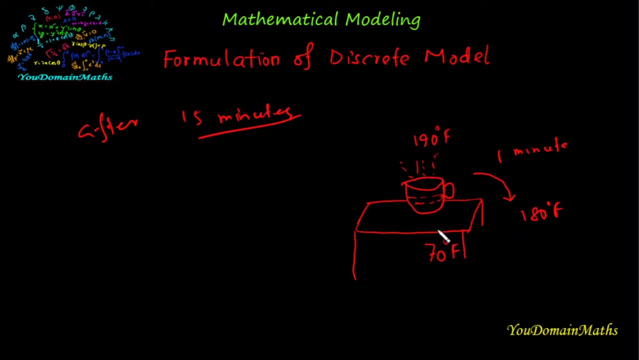 And its own temperature. So mathematically it will be defined such as The temperature Tn plus 1 minus Tn. That means the difference between two time temperature. So this is the rate of change of temperature And which is proportional to the difference of own temperature. 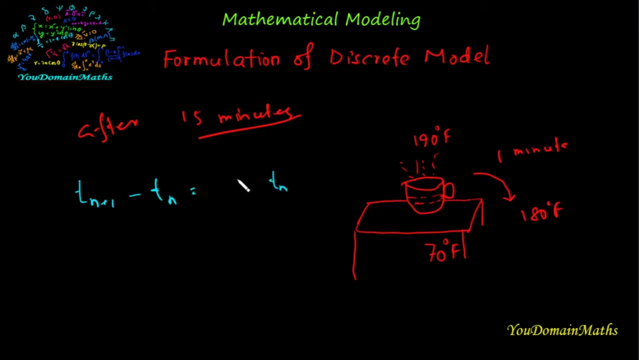 That means own temperature And the room temperature. So K is the proportional constant. This is the mathematical model According to the Newton's law of cooling, Part Tn with the temperature of coffee after N minutes And S is the temperature of room. 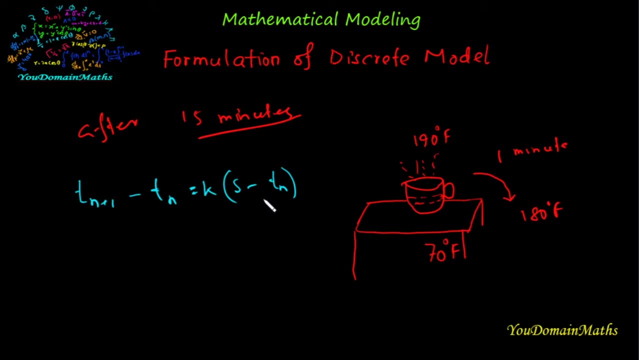 So S minus Tn The difference between Own temperature and Temperature of its surrounding, And Tn plus 1 minus Tn Is the difference While Difference between two time Time temperature. So difference between temperature at two times. 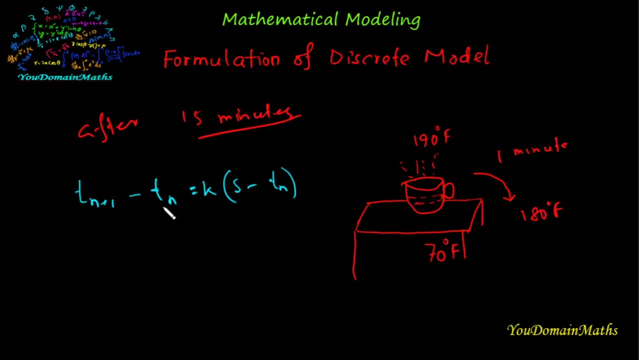 Firstly, we use the Given information. Suppose, After one minutes The temperature is 180 degree Fahrenheit. So this is T1. Because the initial Temperature T0.. So after one minutes The temperature is T1.. 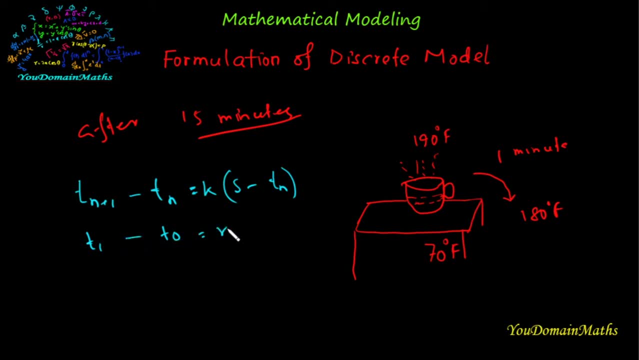 So this is T1 minus T, Equal to T into S minus T. This Rule Applied for The given Chapter, So 180.. That means After one minutes The Temperature of coffee Is 180 degree Fahrenheit. 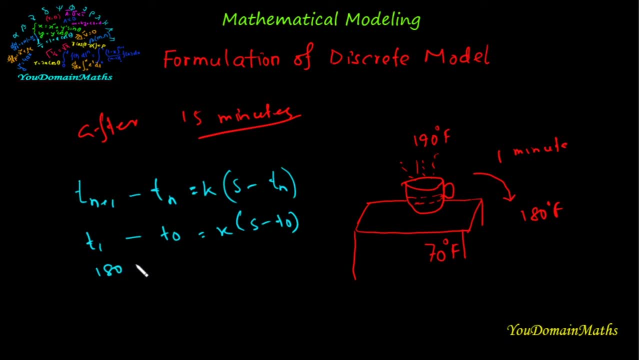 And initially It was 190.. So The temperature Of coffee Is 180 degree Fahrenheit And Initially It was 190.. So The temperature Of coffee Is T0.. So The temperature. 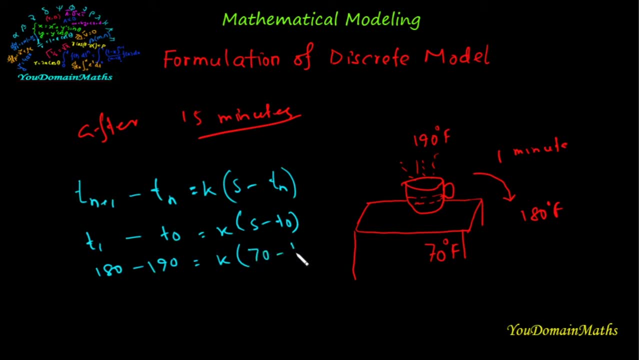 Is 180 degree Fahrenheit And The Initial Temperature Is 190.. So Find The Values Of K Equal to One By 12.. If We Putting These Values, 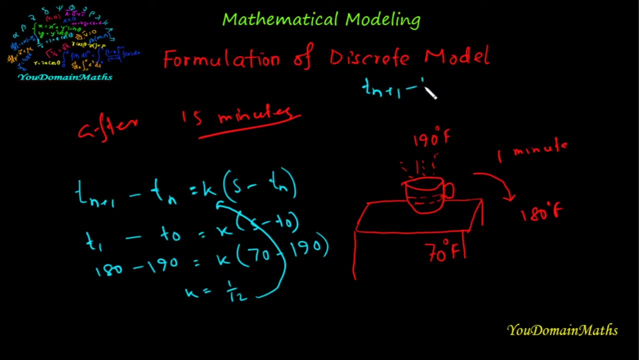 In The P N Plus One Minus TN, Equal To One By 12. S. Now We Find The Temperature At After 15.. So This: 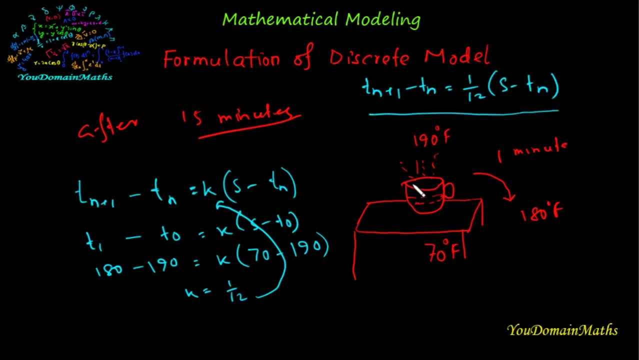 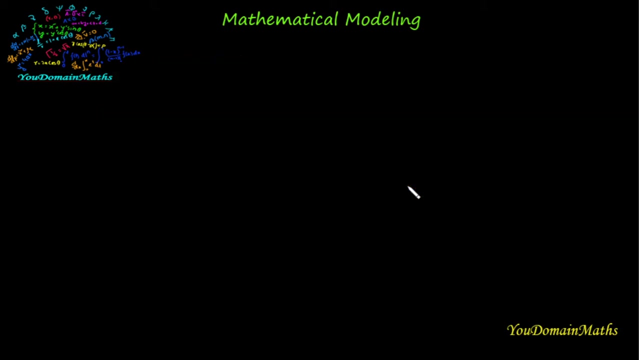 Is The Speed Model. Firstly We Solve It fitting the values of n equal to 15. then we will find the compressor after 15 minutes. firstly we solve it so the model tn plus 1 equal to tn plus 1 by 12, 70 minus tn. 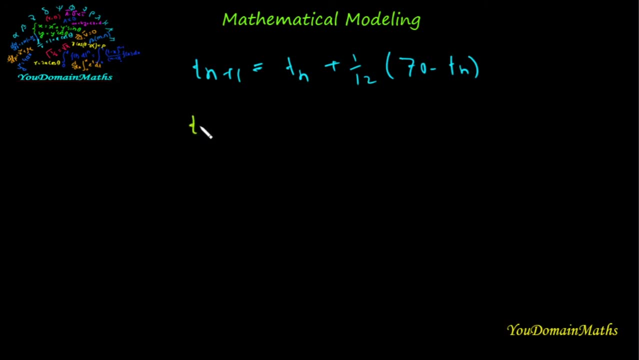 so the equation rearranged as this way: and this the equation of a linear discrete model. so when we solve it, then we'll find the nth temperature. that means after 10 time minutes. what's the temperature for solving this discrete model? please? for the previous video on the lecture, the 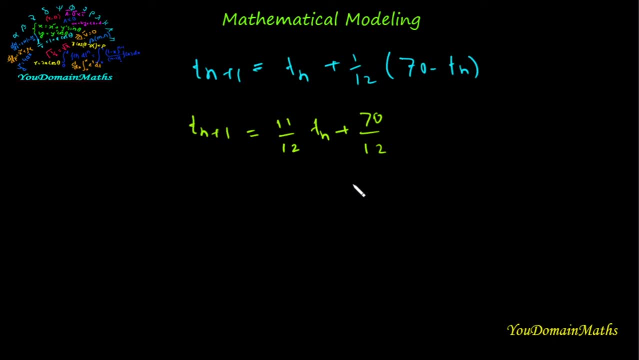 linear, non-homogeneous. first order, discrete product section, which was discussed in previous. so now we will write only the solution of this first order: linear, non-homogeneous. this is the solution. equation: tn equal to 11 by 12, n. 190 plus 70, 1 minus even 12 and n. that is the second bracket. 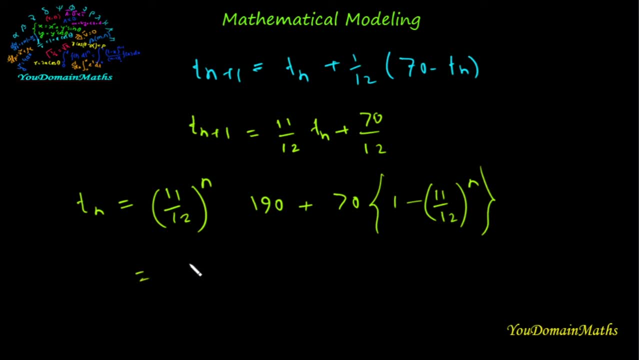 used and amplifying this, then we get 70 plus 1, 20,, 11 by 12, N, equal to 0,, 1,, 2, 3, F P N. The initial temperature will be noted by the T0. And after 1 minute it is T1.. After 2 minute it is T2.. And after 3 minute it. 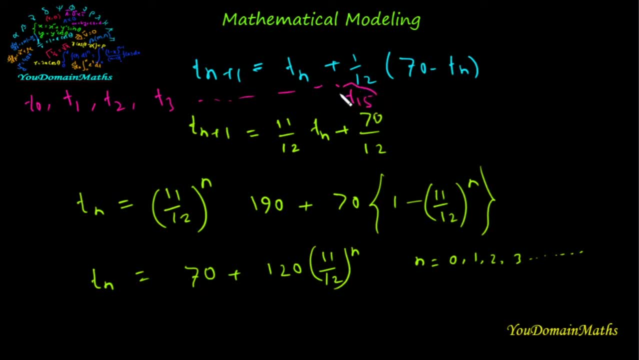 is T3. So after 15 minute it is T15. So putting these values of N in this equation, So when N equal to 15, then we get T15. And the T15, putting these values of T15, then 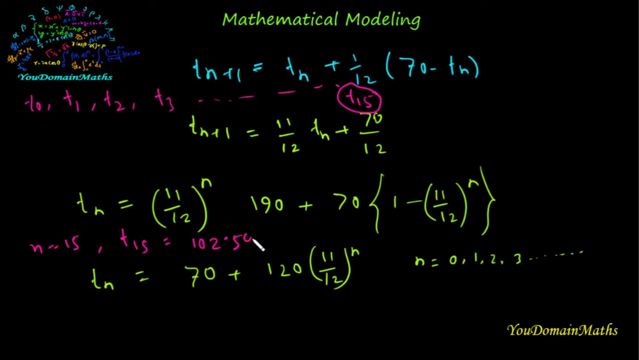 we get 120.54.. So we can say that after 15 minutes the coffee has cooled to just under 120.54 Fahrenheit. for picture Now we will discuss another simple model. Suppose TN with the temperature in degree. centigrade must be N, with the number of meter above on the ground. That is the ground. 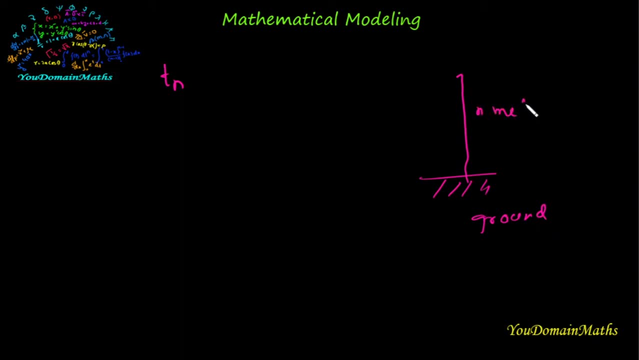 And N meter for is the temperature. The air cools by about 0.02 degree Celsius for each meter rise above the ground level. So repeat this: The temperature in degree centigrade and N may be the meter above the ground And the. 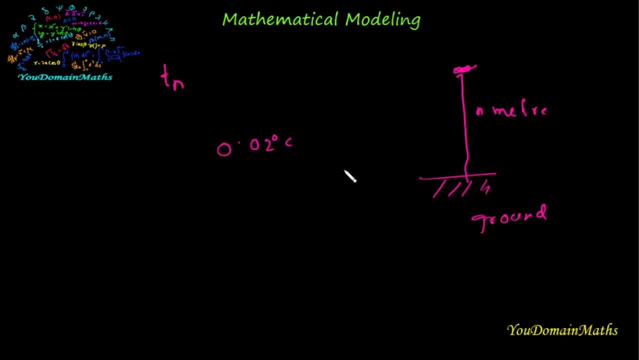 air cools by about 0.02 degree Celsius for each meter rise above the ground level. Formulate discrete dynamical model to solution or find out its situation. TN: with a temperature it will be different on the previous temperature. That means: 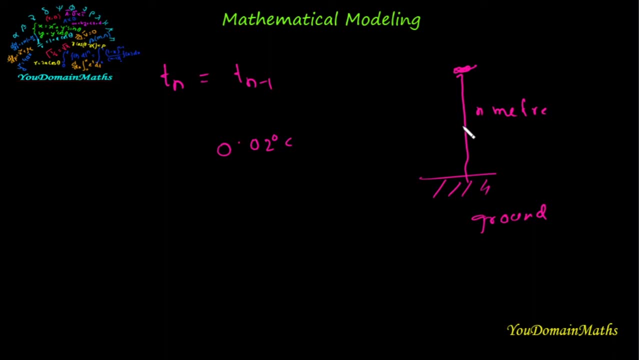 N minus 1 meter height. At this level the temperature is TN minus 1. And the temperature is decreased 0.02 for every meter. So this is the discrete model. The present temperature will be different on previous temperature And the previous temperature. will be different. on input power, This time we will use the return on break and that we set at this point, given continuous state temperature. So the current temperature, which is 0. tenho select on the previous temperature And to get TN will depend on TN values. So 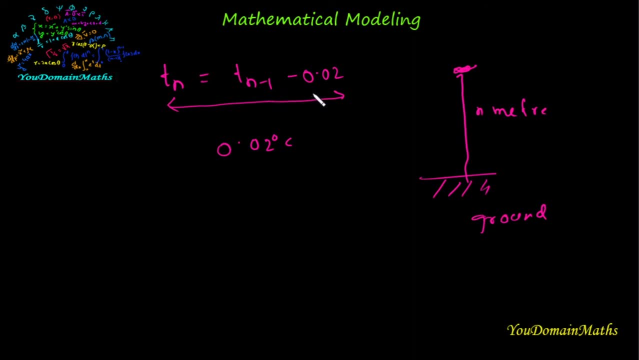 previous temperature minus 0.02 degree Celsius, because the air cools by about 0.02 degree Celsius for each meter rise above the ground level. when we solve it, then we get the Tn equal to T0 minus 0.02 m and we can. 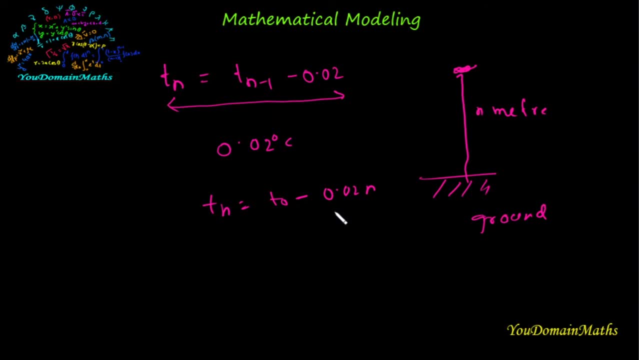 say easily if the temperature at ground level is 30 degree and find the temperature above the 500 meter. so putting these values in the values of n equal to 500 and T0 equal to 5, and putting these values and we get so easy the values of Tn.